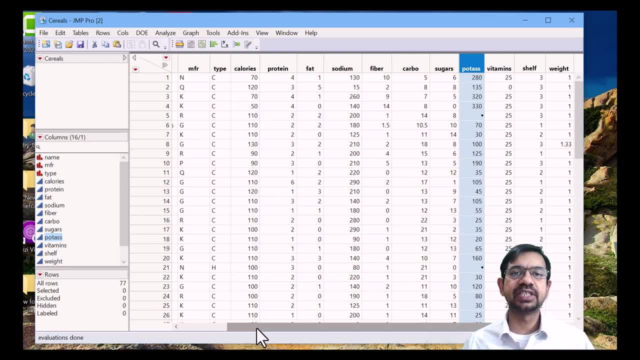 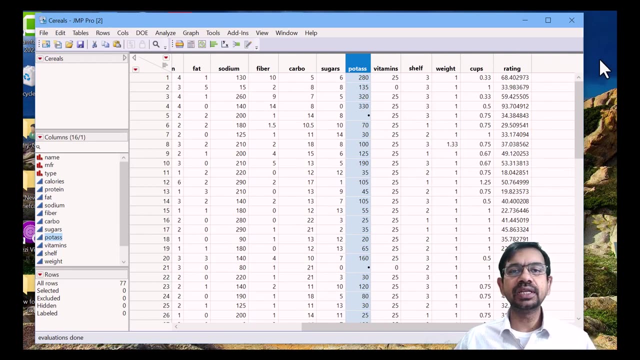 contained in these numerical variables into a smaller set of variables. So to motivate the idea behind principle component, let's work with two variables. Suppose we want to combine calories and ratings into maybe one new variable which will capture bulk of the information contained in these two variables. So 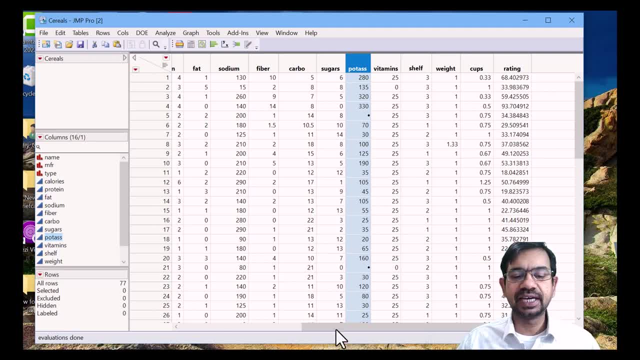 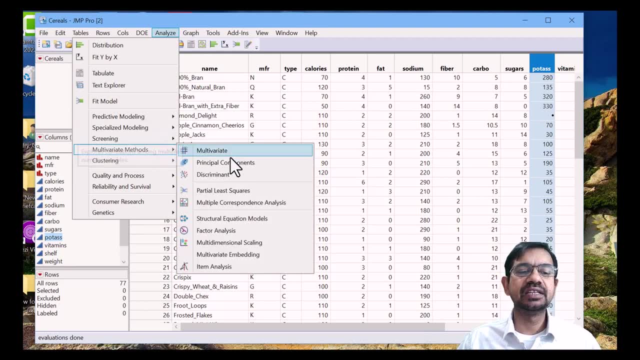 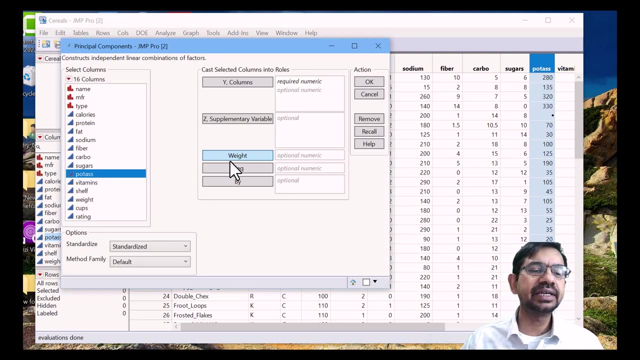 The method we will use for this is the principles component analysis. To do that we can go to analyze then multivariate methods and then principles component. Then we include our Y variables that we want to combine. So in our case we want to combine. 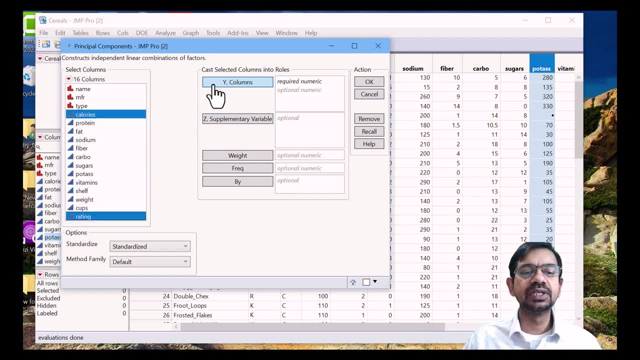 calories and we want to combine ratings, So I'm going to move them to our Y Now, just to illustrate. the default is that all these variables are converted to Z scores or standardized. Let's say that we want to just have unscaled, Unscaled. 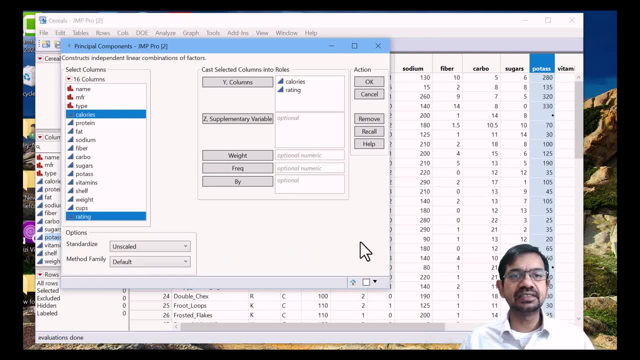 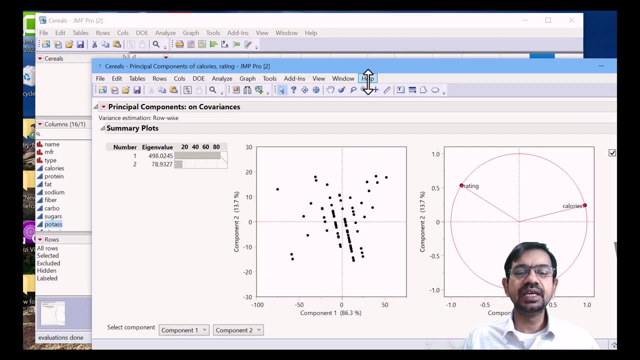 would mean that they're not divided by the standard deviation, but they're still centered. It means that they're subtracted by the individual means. So then we click OK And this is our output. So here we see that because we have two variables, we can at the 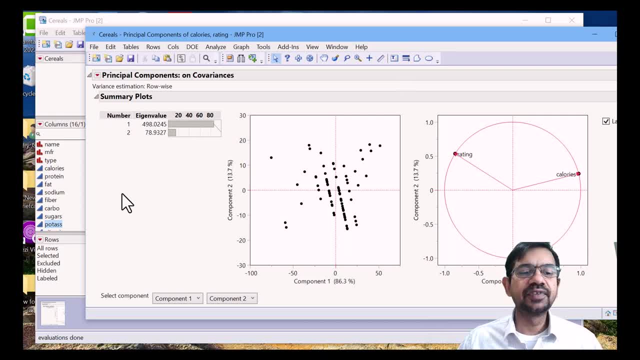 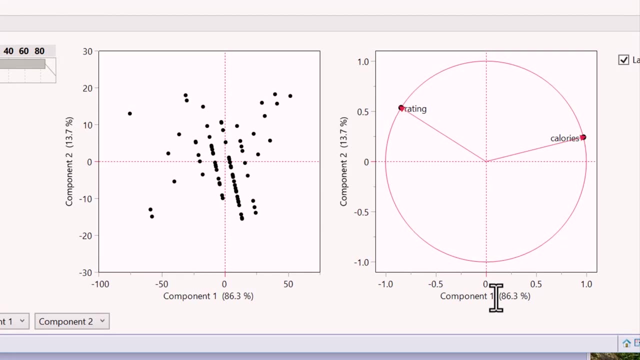 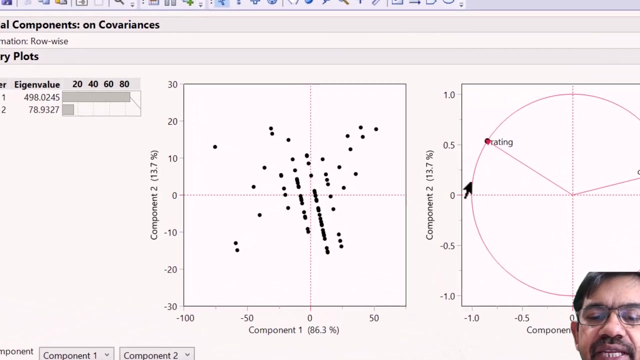 most create two new variables from them. The first variable that we create has 86.3% of the variation, As we can see here that component one has 86.3% of the information contained between ratings and calories, and component two picks up the remaining 13% of. 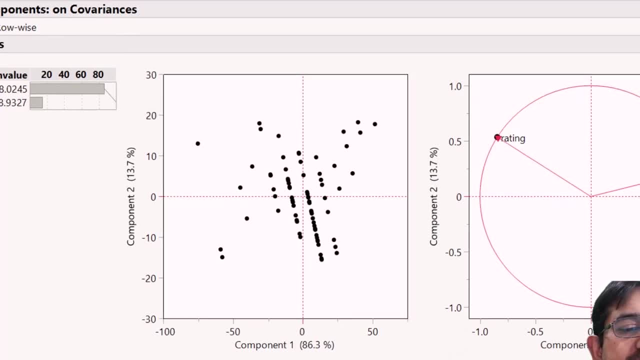 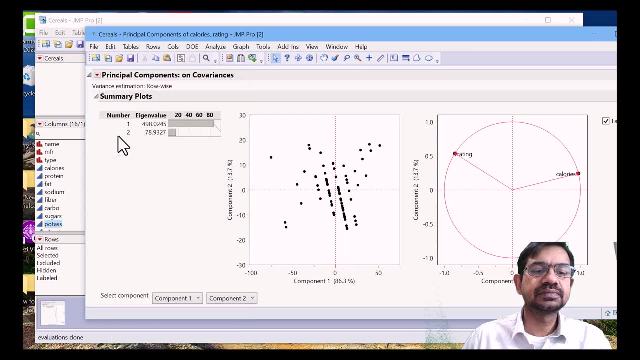 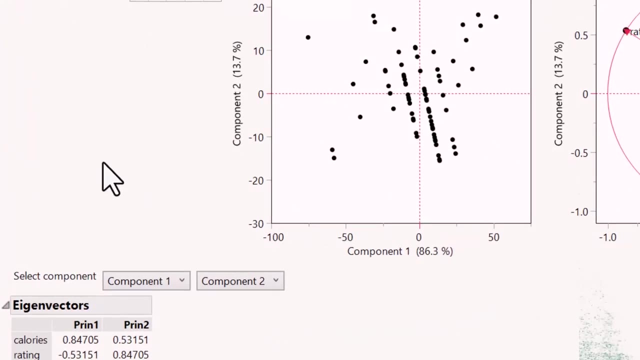 the variation. We can also look at these in detail. I'll click on the little red arrow and I'll click on eigenvectors. Eigenvectors show us the weight that each of these variables has in each of the components. So in the first principal component, rating calories will enter with the weight of 0.84. 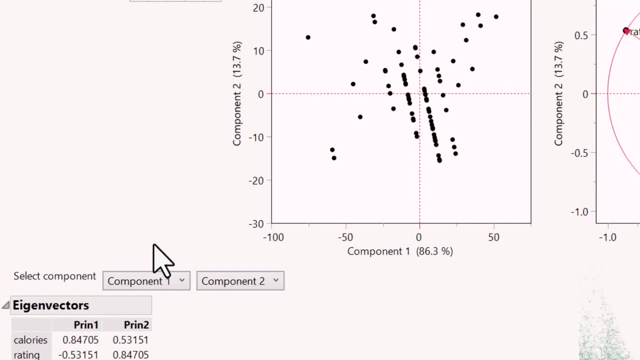 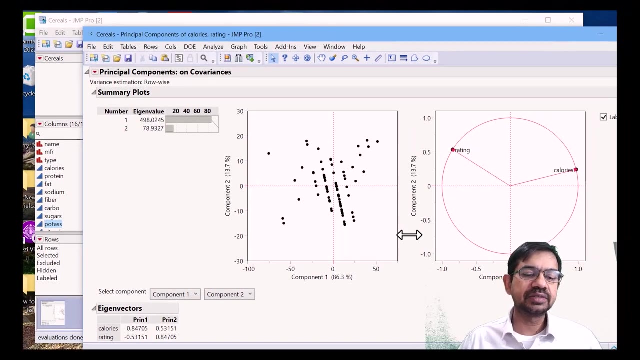 and ratings will enter with the weight of minus 0.53.. And then the second principal component: calories enter with the weight of 0.53 and ratings enter with the weight of 0.84.. Now, what does that mean? If I were to create a new principal, a new variable for component one, I would, for the 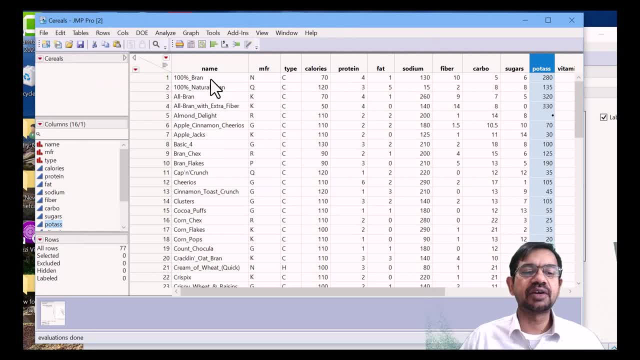 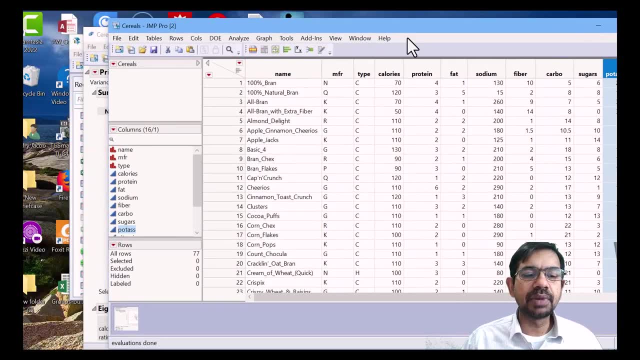 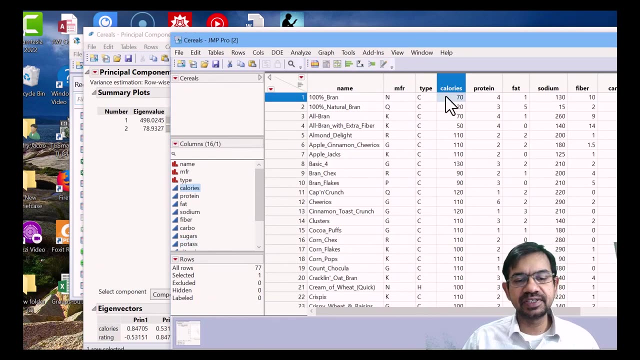 first serial, which in this case is 100% brand. I would construct this by multiplying my weight, which we said was 0.847, with 70 minus the average calories in my data set, And then I would Add, or in this case, minus 0.53 times the rating score, which is 68.40 minus the average. 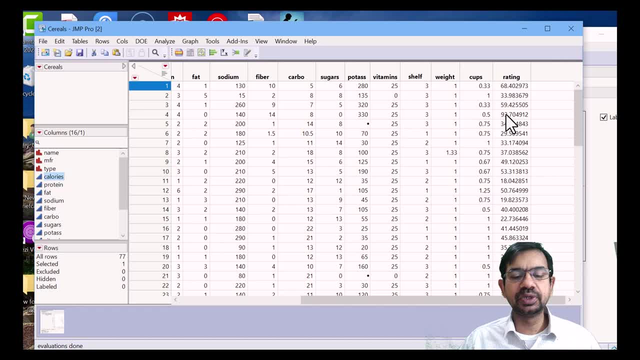 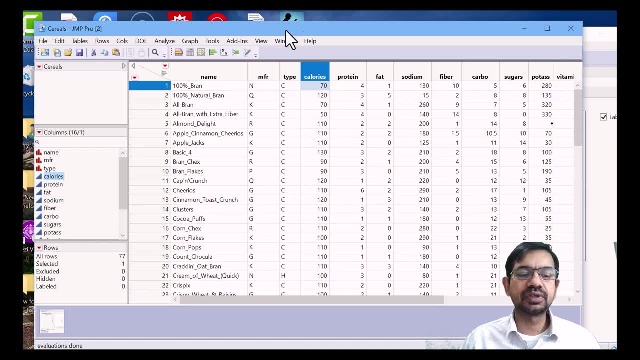 rating. So this would be my first component, And I would keep doing that for the second and the third serial and so forth. So in the second serial we would do 0.84, which is what we have here, times 120 minus. 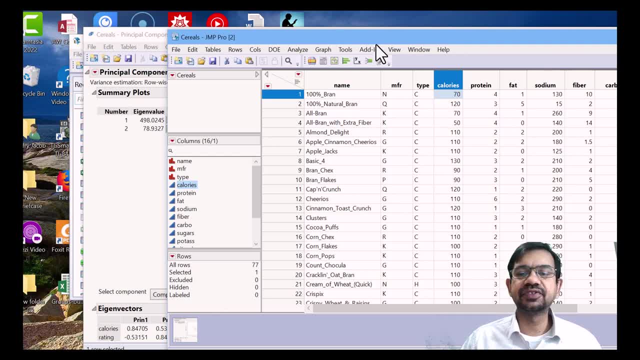 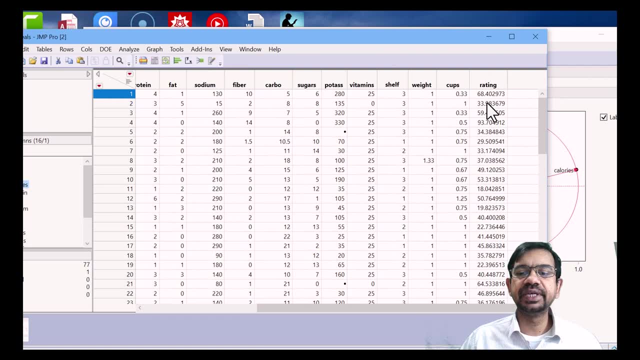 the average calories And then minus 0.53.. Okay, And then we look at the value of ratings for the second serial, which would be 33.98 minus the average rating score. So this is how we construct the first principal component. 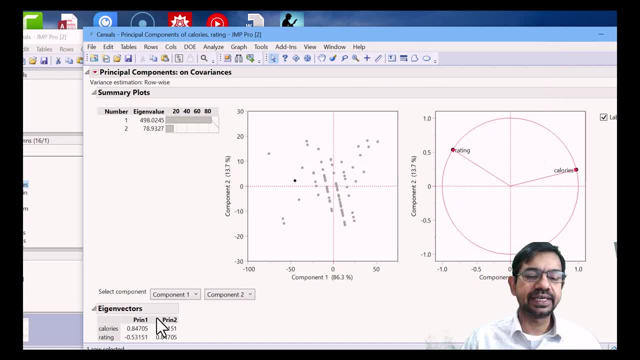 And then, similarly, we can construct the second principal component, applying these respective weights to our serials, Another way in which we can see how much information in our data set, which in this case is calories and ratings, is contained by these principles. 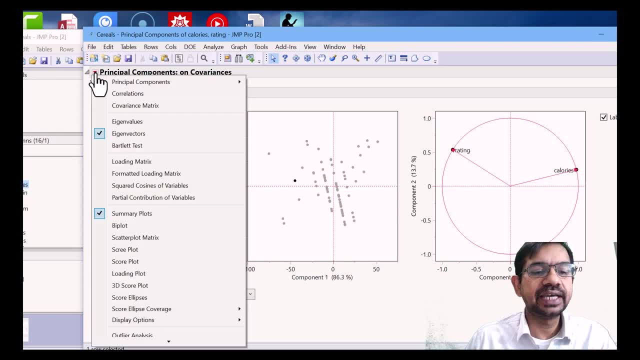 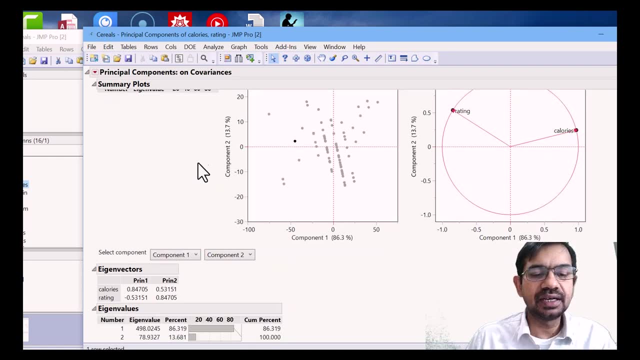 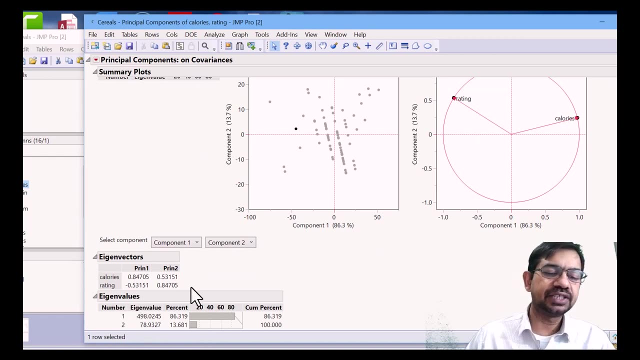 Principal component. We can go to the little red arrow, And then this time we'll request eigenvalues, even though we got them with our result as well. This kind of gives us more clarity. So let's say that the total variation between these two principal components is the sum. 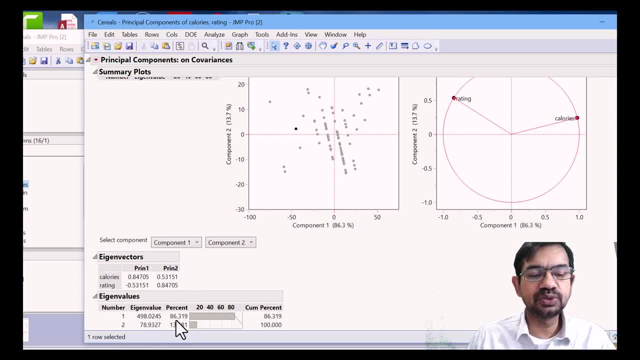 of these two eigenvalues of this principal component One is capturing 86.3% of the information that the data contains. And then This principal component is capturing 13.68% of the information contained in the data. So if we were to include just component one, we would synthesize calories and ratings into 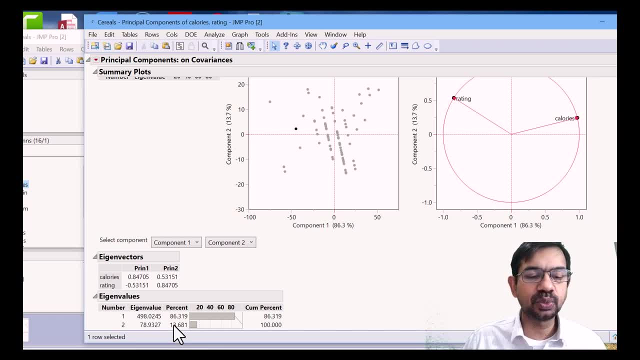 one variable, let's say, and that one variable we choose is component one, then we would be capturing 86.3% information contained in the combination of these two values. Now, Why? Why couldn't we have just chosen one of those two instead of creating this new principal? 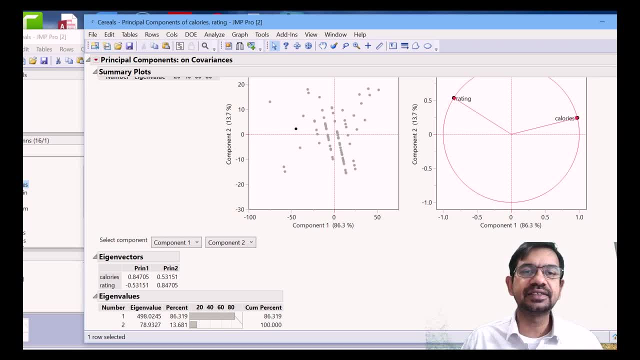 component. Well, to see this, we can see how much total information is captured by each of these individual variables. So, to see that we can look at the covariance matrix To obtain the covariance matrix between ratings and calories, we can go to analyze multivariate. 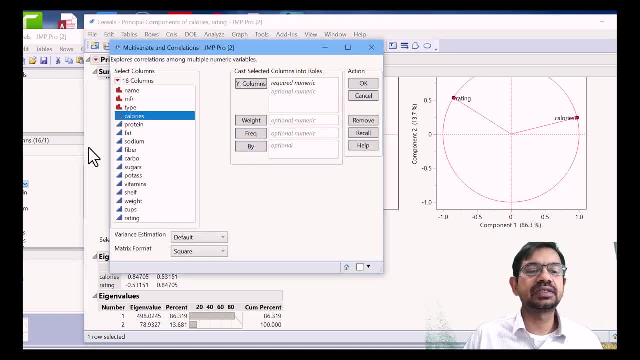 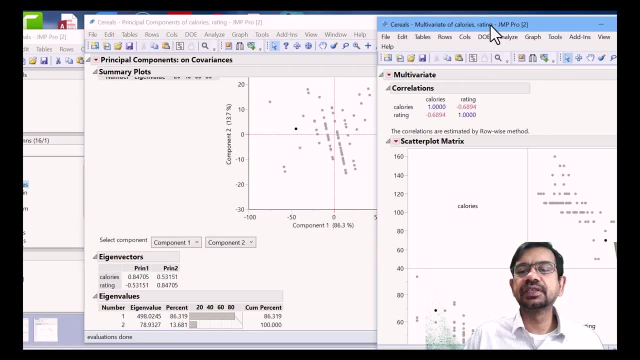 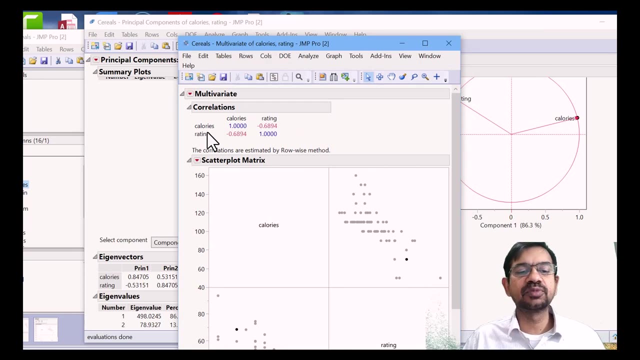 methods, Multivariate this time, And then We can assign our calories and ratings to our y. It will give us the correlation coefficient, which is not the covariance. Correlation coefficients are derived from covariance. To obtain covariance, we can again click on this little red triangle and then click on. 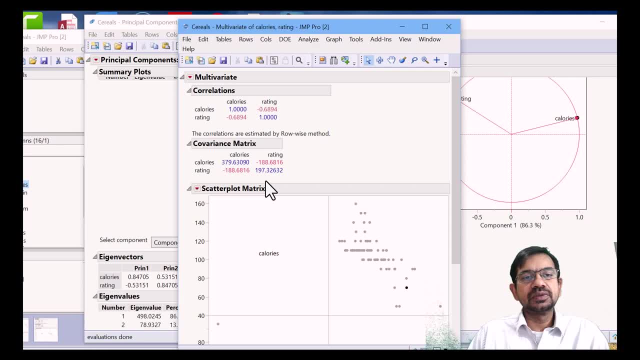 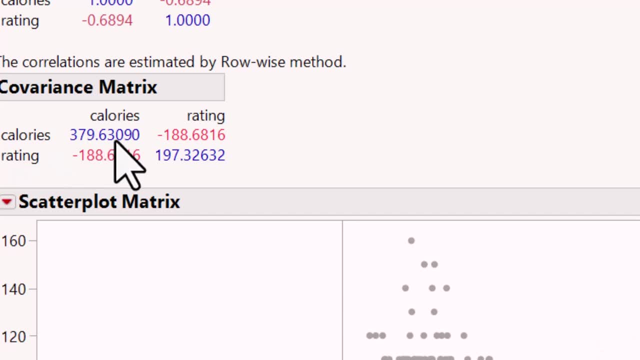 the covariance matrix. So what this tells us is that the variance of calories is 306.5.. So The variance of calories is 379.63.. And the variance of ratings is 197.32.. So the total variation in our data is 379.6 plus 197.32.. 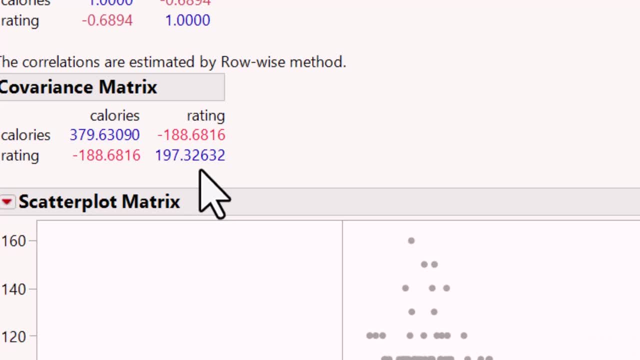 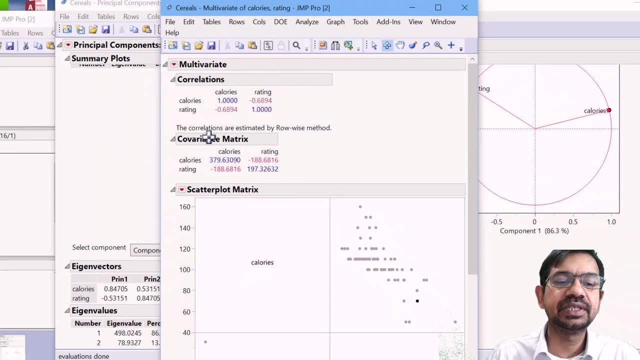 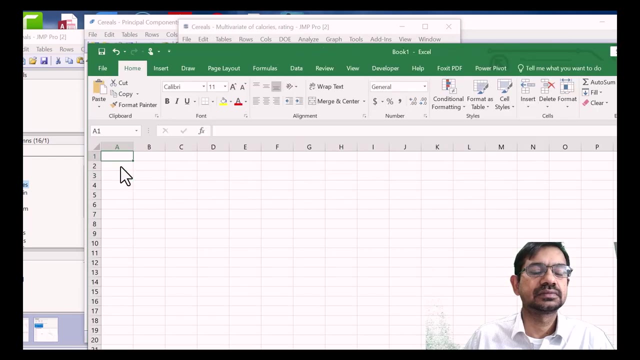 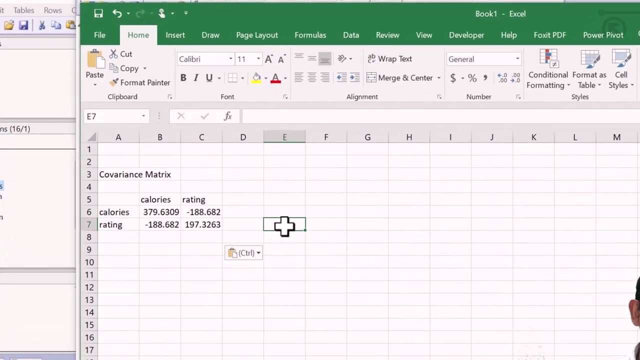 And then we can now calculate the share of each of these individual variables in our total variance. We can bring this into Excel, So I'll just copy this table And then Move it in Excel And then to see the share that calories is in the total variation, in the data we can. 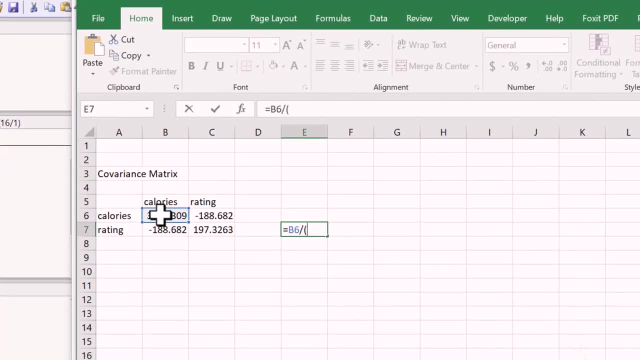 do a simple calculation where we divide the variance of calories with the sum of the variance of ratings and calories And we get that Roughly 60% of the variation in the data set is accounted for by calories, which means that one minus. 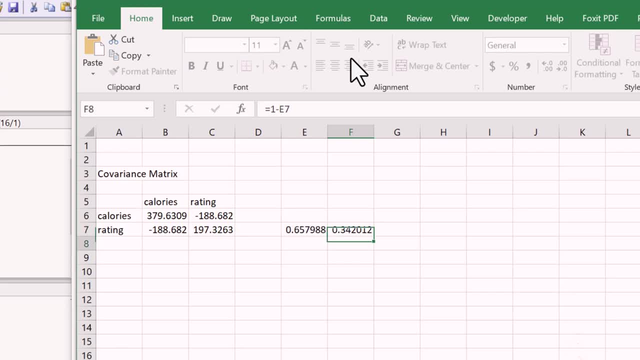 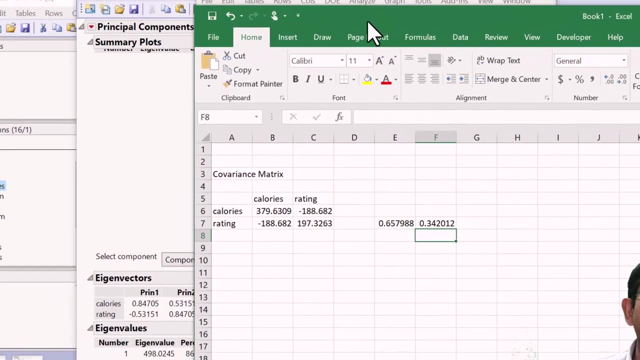 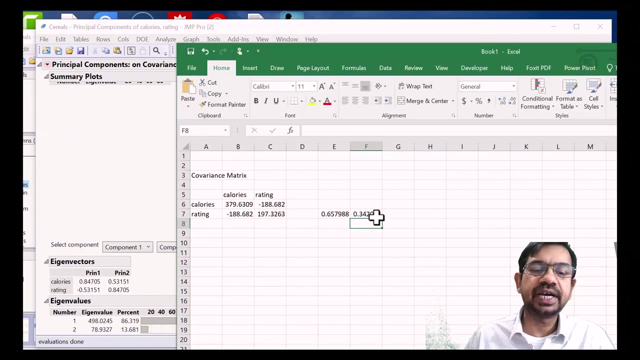 this is accounted for by ratings to 34%. Now, if we were to include either calories or ratings, then we should be including both of them. Then what we are doing is that we are only capturing either 65% of the information, or 66% in this case. 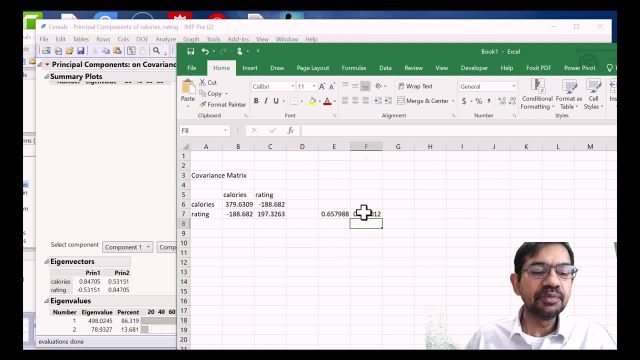 Or only 34% of the information in our data set. But if we use the principal component that we created, and if we were to use just one of that component, then we would be capturing 86.3% of the variation. So principal components is a better way than to arbitrarily choosing one or the other variable. 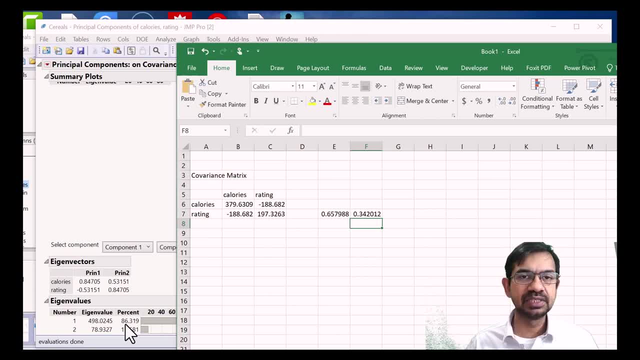 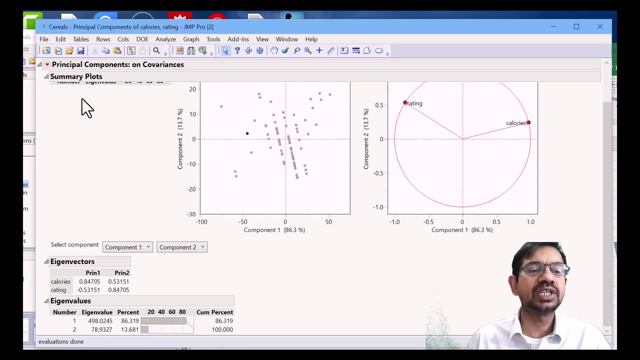 where we're able to distill the information contained between these two variables into one variable, which is essentially a linear combination of these two. Now, how do we generate this for the data set? We had talked about the method to do it individually, but we can do that in jump for the entire data. 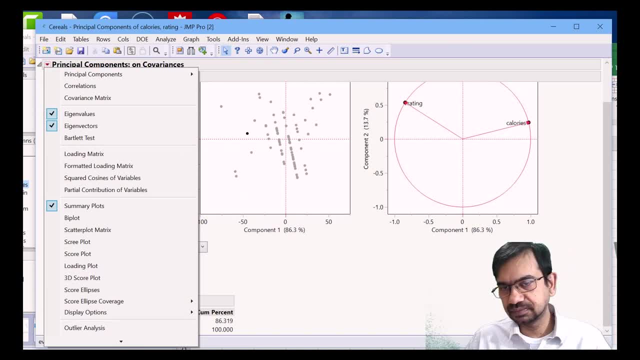 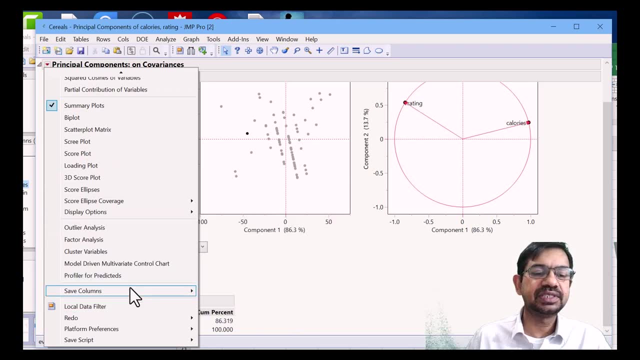 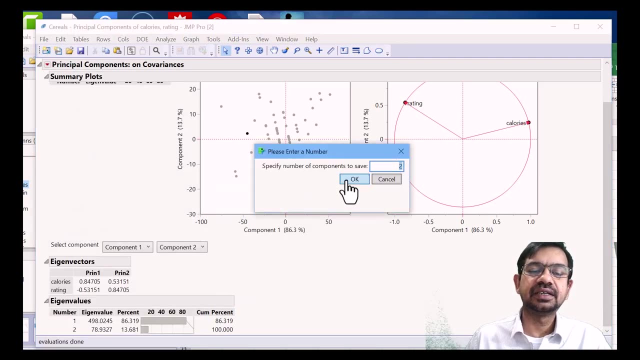 set. We go save columns and then we say save principal components, And in this case we can just save two, And then we can go back to our data set. And then we can go back to our data set Because we have now the number of components generated will be the same as the number of 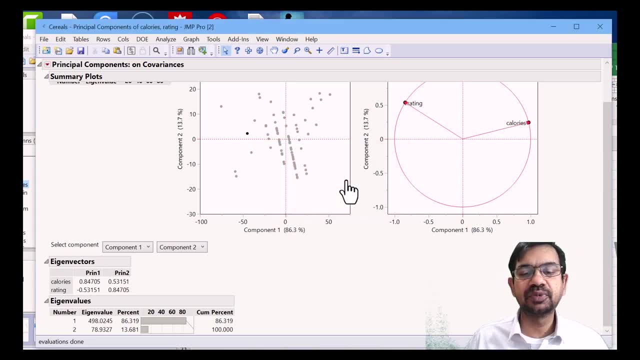 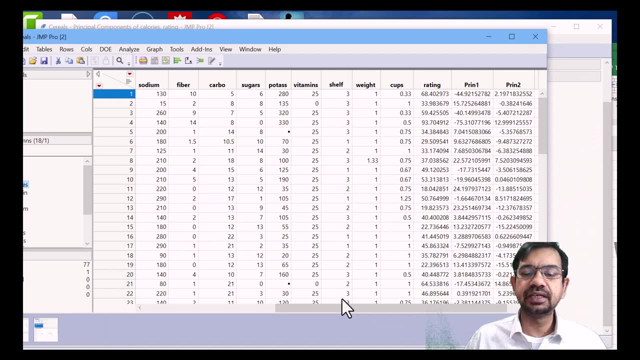 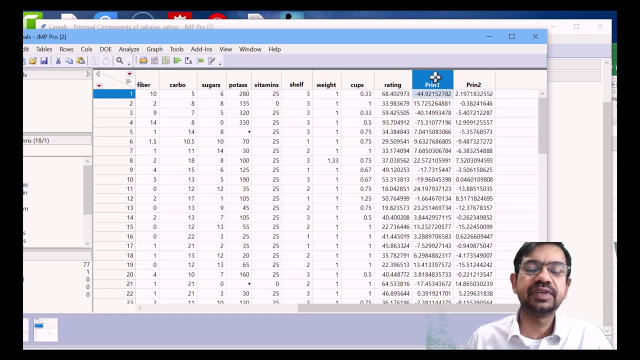 variables we are starting with. So, in case we want to save both our components, we save two. And then, if you look at our data set or data table Here, we have created our component one and component two, So we could just include component one instead of including either rating or calories. 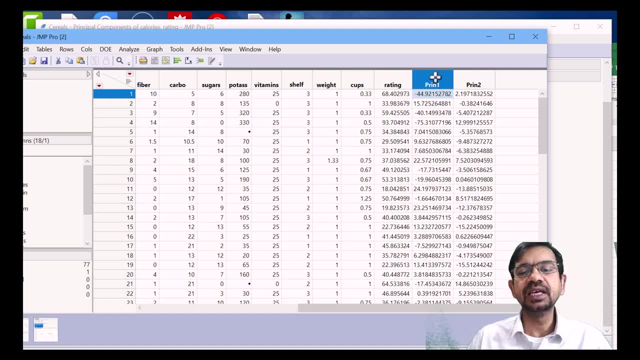 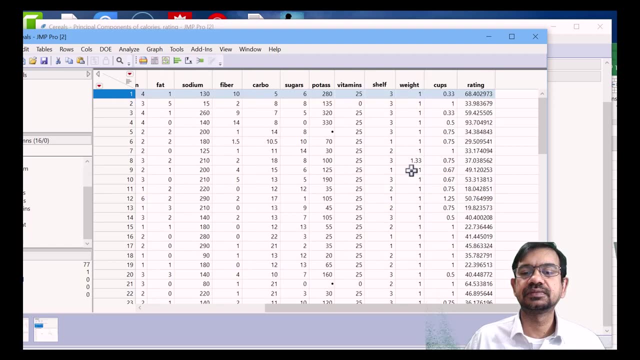 And we would still get, as we saw, 84% of the information. Now this works when we have Two columns, but we can extend this analysis to include all of our 13 columns, So I'm going to Delete these two columns. 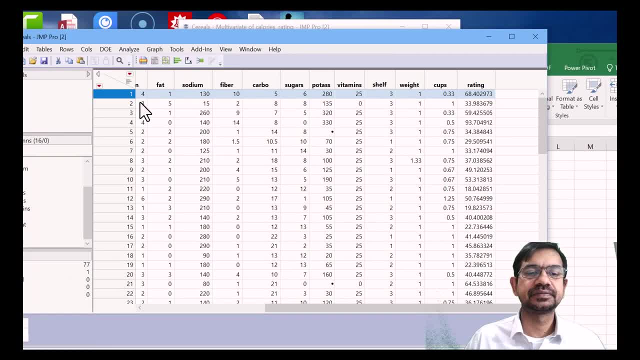 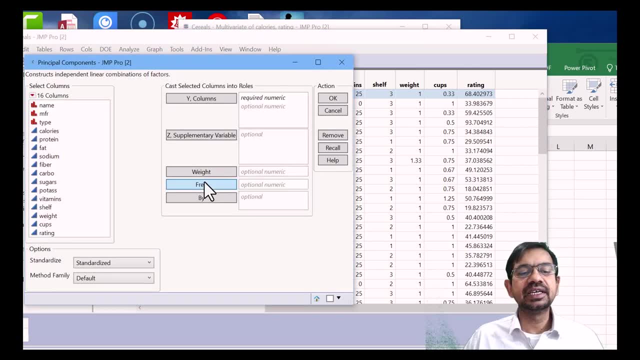 And then we'll start again- Can go to analyze Multivariate methods and principal component, And this time we will include all our qualitative or quantitative variables. We will again Just to Change The process a little bit. We'll work with 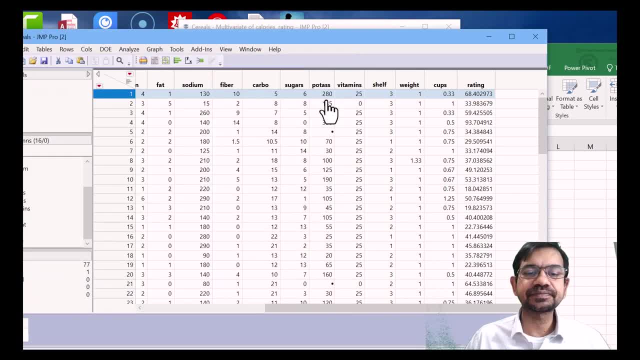 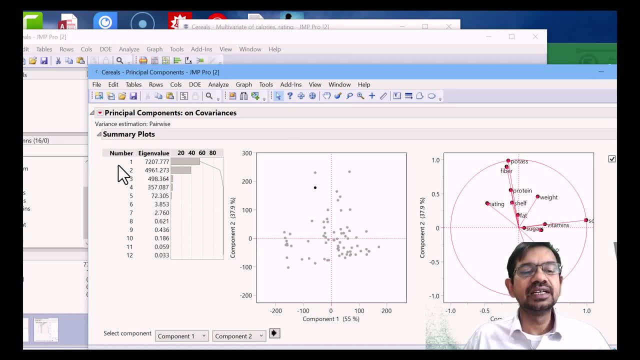 Unscaled instead of standardized values. In this case we get as many components as in the data set. The first principle component that we get, we can see, is capturing close to 60% of the information containing the data. The next one, close to 40, to see these actual. 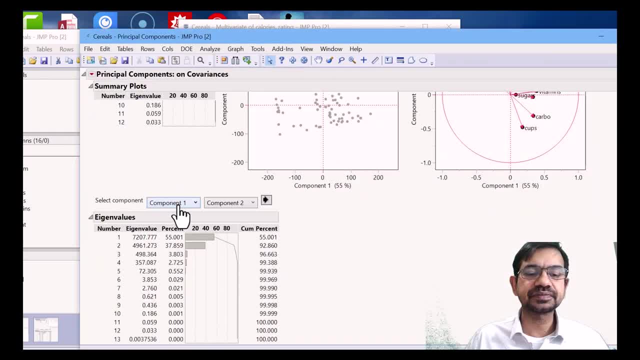 Shares. I can request eigenvalues and we see that the first principal component out of these 13 is able to capture 55% of the information. the second one contributes 37, so cumulatively they both are capturing 92% of the information, the data set and then 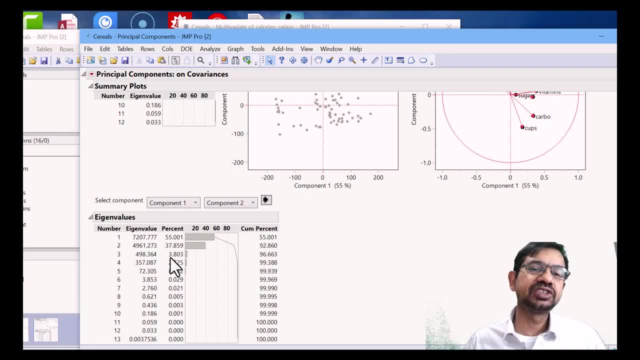 the third one captures additional 3.8. so between the first three principal components we've got 96% of information captured and if you go to four, they've got it almost 99% of the information in the data set. but what are these components and what does it mean by that, so we can see actually how much each of? 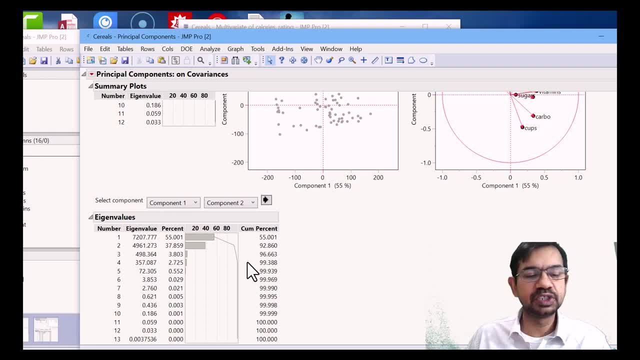 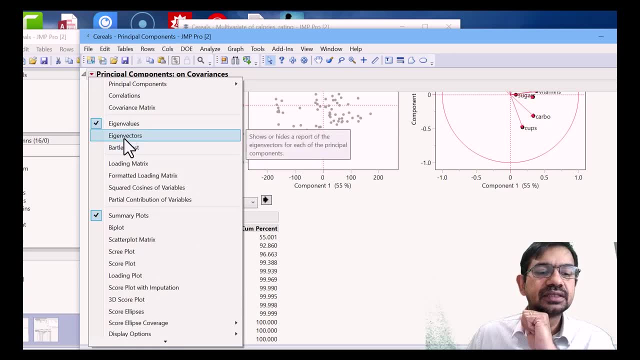 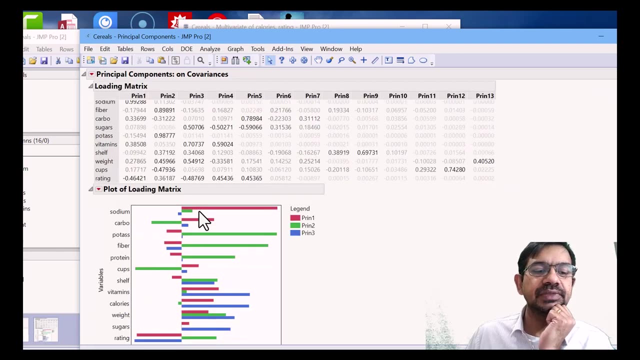 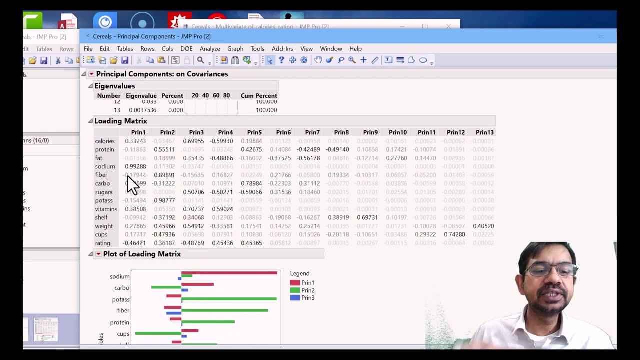 these individual variables contribute to the individual components. and to see that we go to the little red arrow and we can click on the loading matrix, this tells us, for the first principal, sodium is loaded very heavily. so out of the total weight in this, 0.99 goes to sodium. so this is essentially capturing. 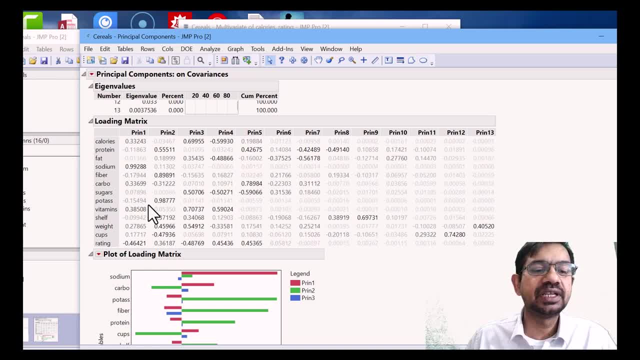 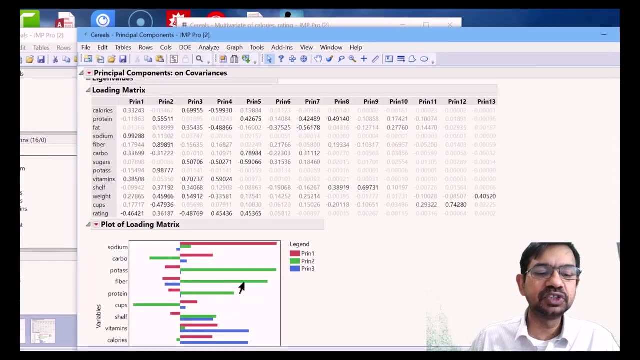 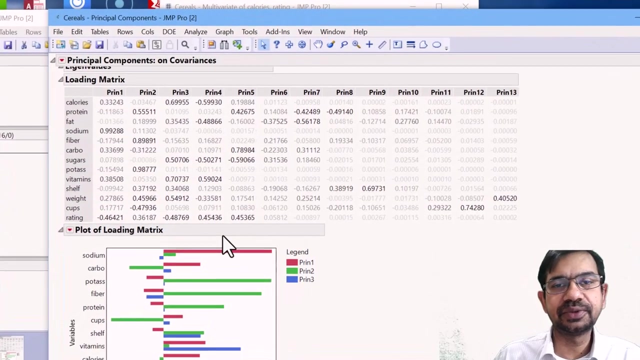 the amount of sodium. the second principal component captures the extent of potassium and then to some extent fiber and so forth. so we can see individually how these components are loading into this. and this is a nice visual tool to see that between the first principal components we see that sodium has the longest red bar. so sodium. 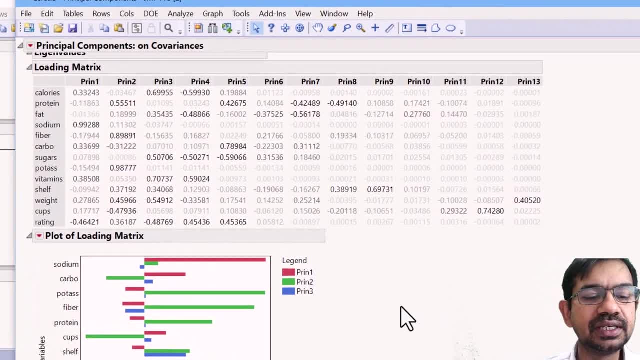 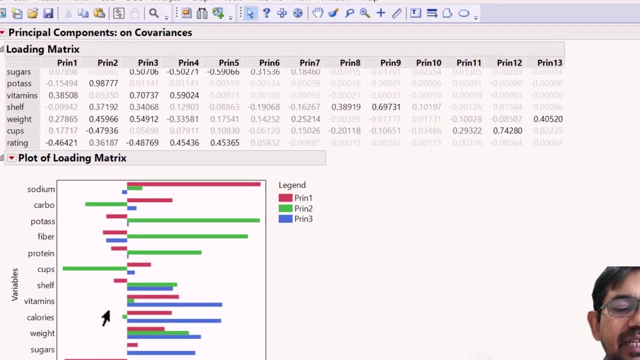 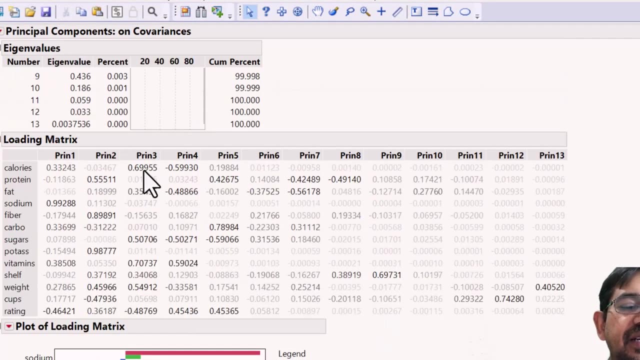 is loading really heavily into component one. component two is put a and then some fiber. rest three is divided in between vitamins, calories, weight and then rating in some ways, and we can see that these are highlighted which are more significant in capturing that. so between them, the largest role is assumed by vitamins. 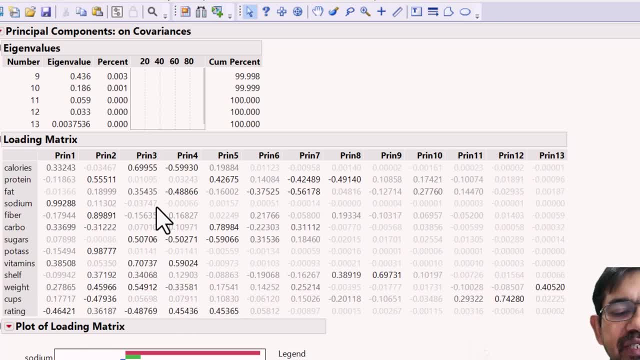 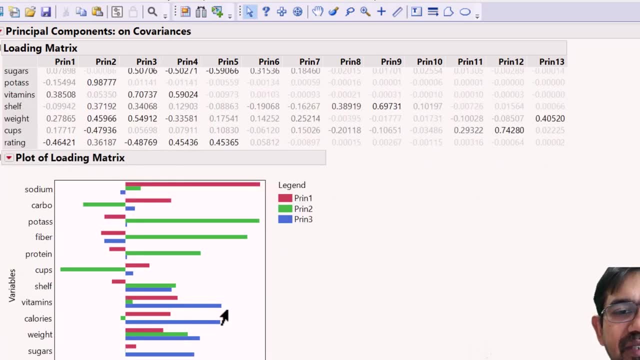 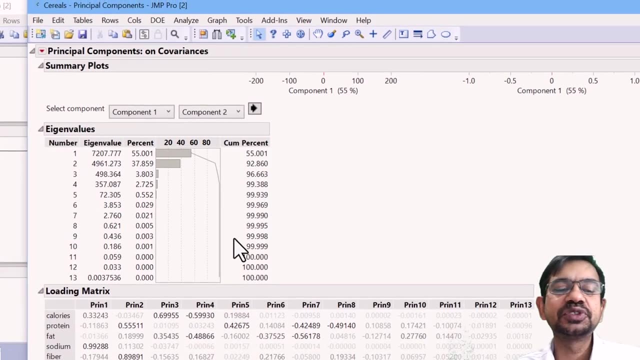 then the next one would be calories. so we can see that in the bar we have for the blue chart we have vitamins as the longest bar and then calories as the second longest and so forth. so if we were to go with this, then we could say that you know what we just need to have maybe the first three. 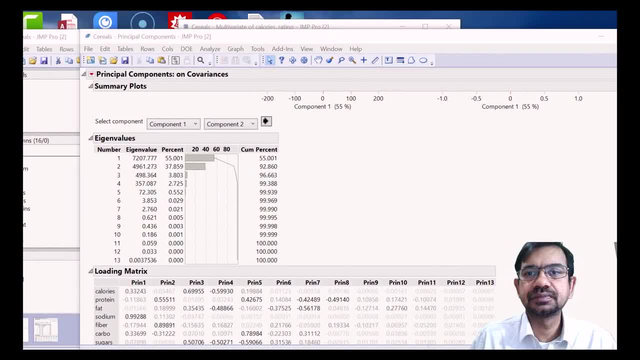 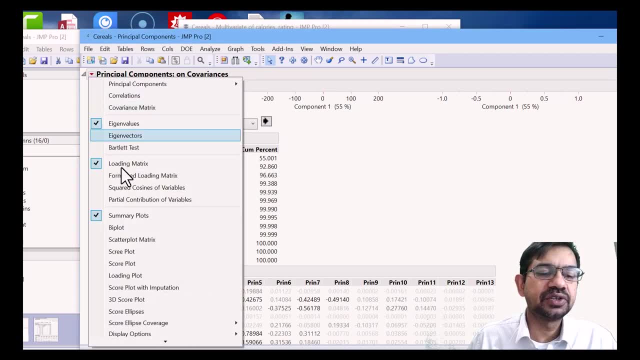 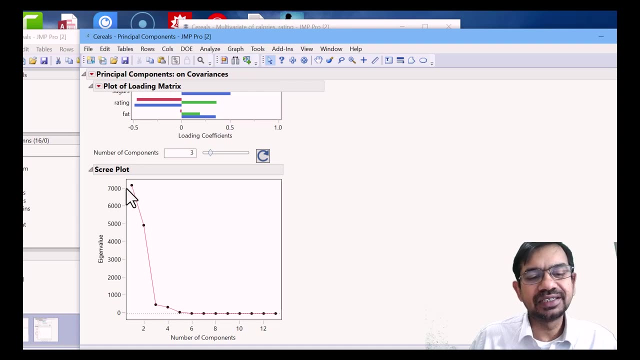 components. and we are done now. this chart that we see is called a scree plot. we can obtain this individually as well. I go to the options and I click on scree plot. so this is like an elbow chart in some ways. typically would include components after which, if you were to think, 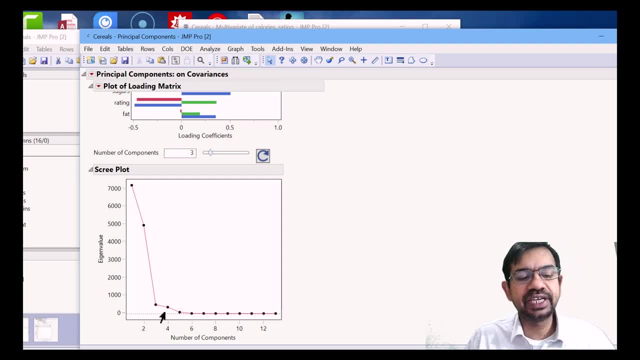 of this as an elbow. the elbow kind of becomes straight after this. this is the elbow joint. so even including the first three or four components would capture bulk of the information in the data set. now, does that mean that, yay, instead of 13 we just need three or four? well, as I said, we did a little bit of cheating here. if you look at the data set again, 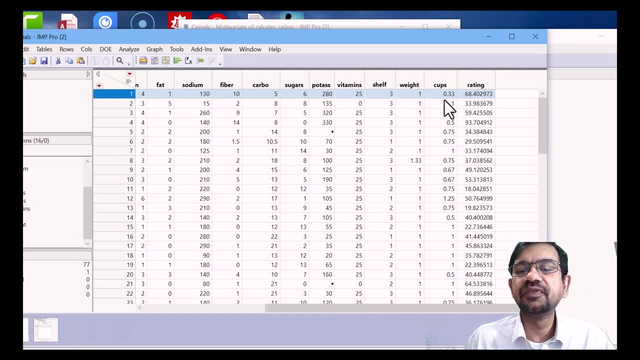 we have these data sets on disparate scores. we have weight, which is essentially an integer one, and then we have sodium, which is in milligrams, and it is, it ranges from 220. so contrast the scale of, you know, these numbers which are in hundreds. so is potassium, along with some other. 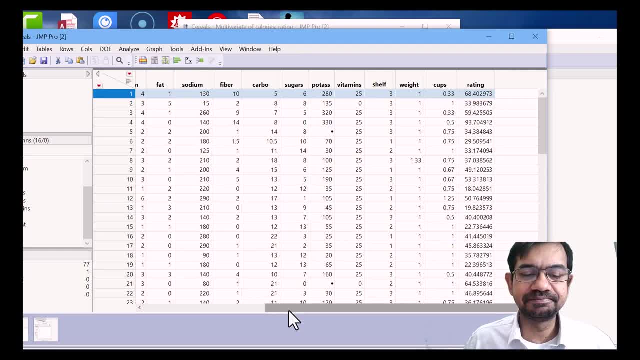 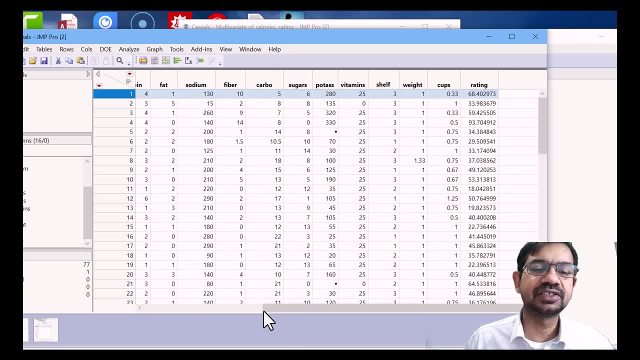 numbers which are in tens. even so, this is not really a balanced way to approach this combination of data set, where sodium and potassium, unsurprisingly, are driving a bulk of this information. to guard against that, we would standardize our variable. so we'll contrast and see the difference that standardization 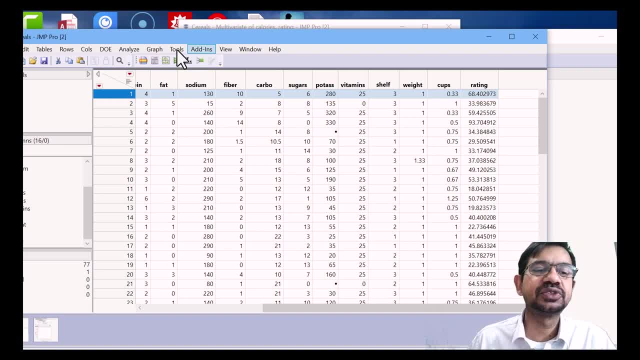 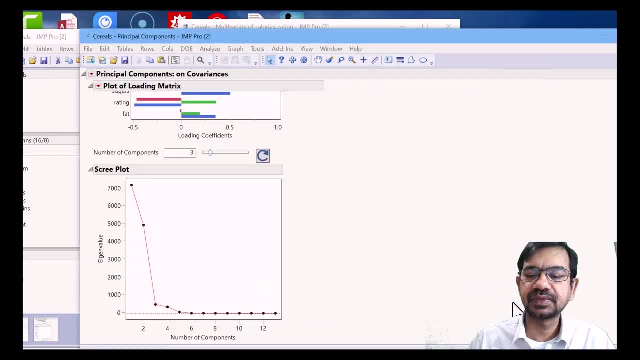 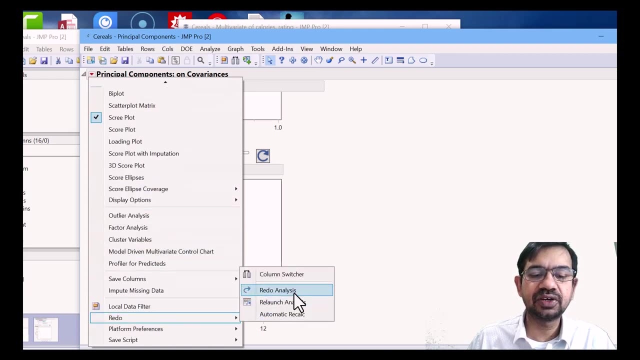 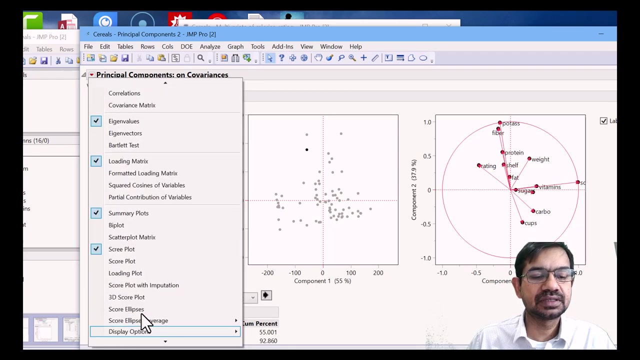 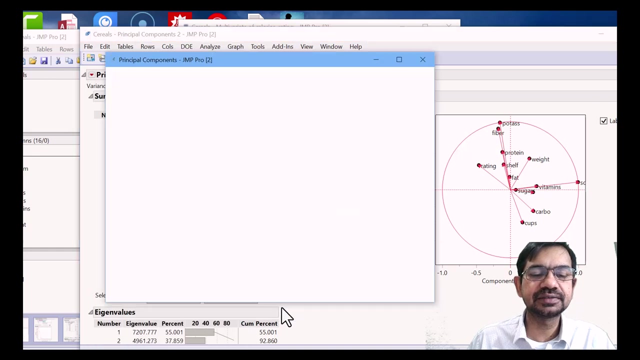 makes in capturing information from our data set. so here again we could analyze or we could go back to our old result, and here we can click on redo analysis and we click on relaunch analysis. it opens the you we can click on redo and you can click on relaunch analysis. this will open up. 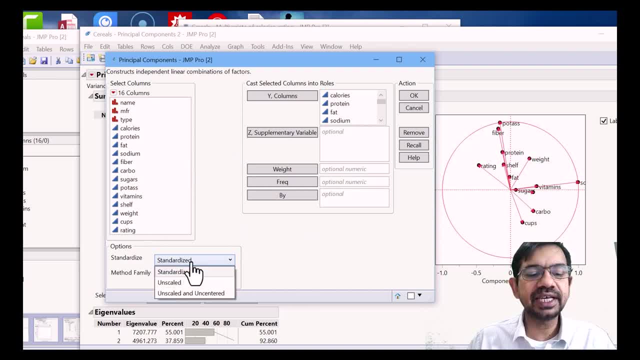 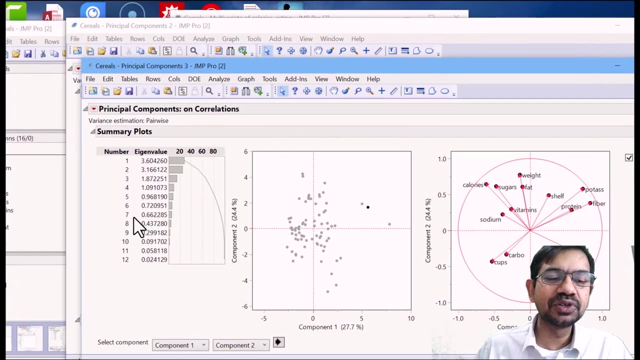 the initial dialog box, but we will now let our data be standardized, so converting to z-scores. we'll leave this checked and we won't change this. and now let's generate the principal components. and here we see that we have to go fairly far into our components to get most of the.